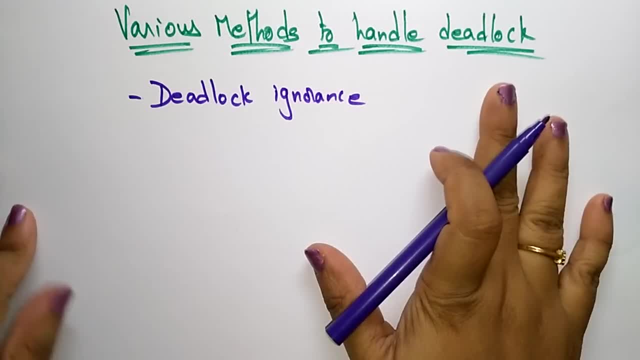 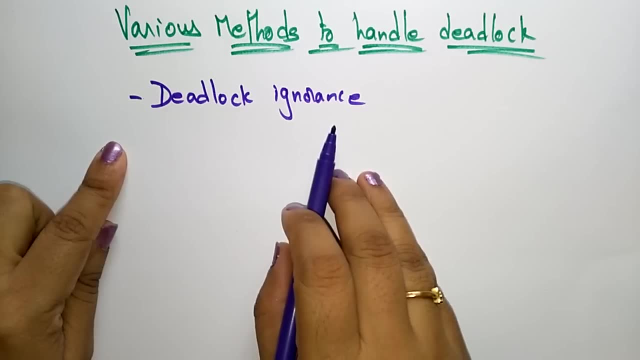 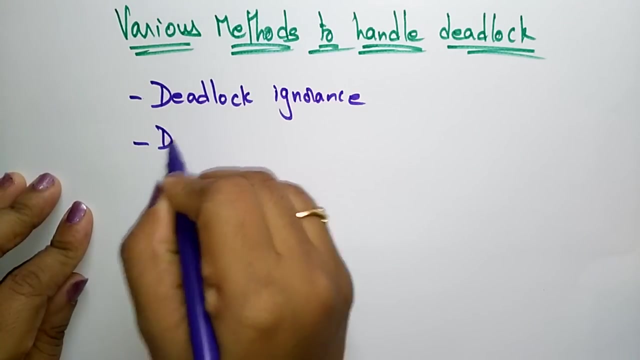 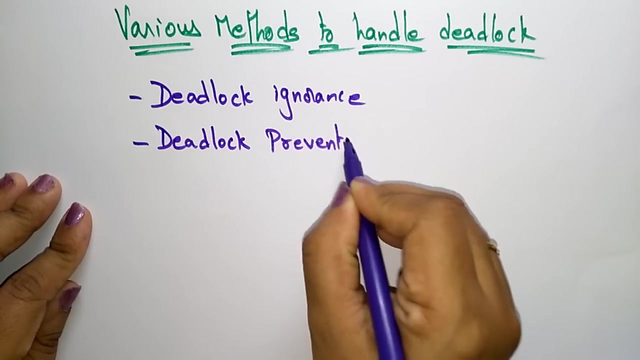 Hi students, coming to the various methods to handle the deadlock, There are different methods to handle deadlock whenever it is occurred. So the first thing is deadlock ignorance, If you want, if you just ignore the deadlock if it is occurred. that is the first solution. And next solution is it's better to prevent the deadlock before it occurs. That is the deadlock prevention. So prevention is better than the cure. So better you just prevent the deadlock before it occurs. 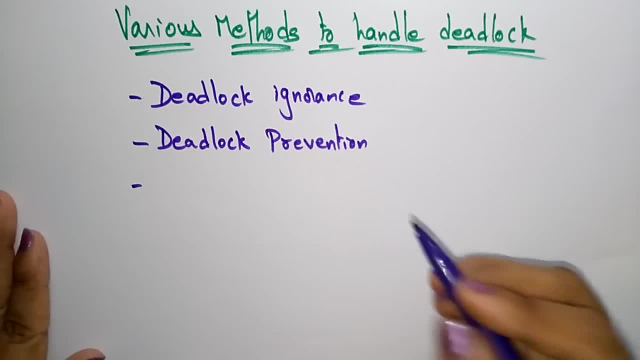 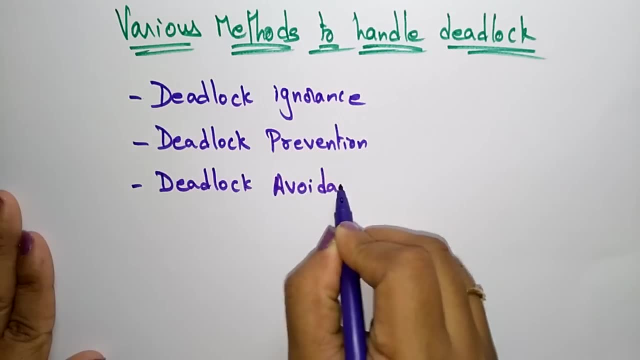 Before it is occurring. And the next method to handle the deadlock is it's better to avoid the deadlock, Deadlock avoidance, Deadlock avoidance and the final is the deadlock detection and recovery. Detection and recovery. So these are the various methods to handle the deadlock. So first thing is: 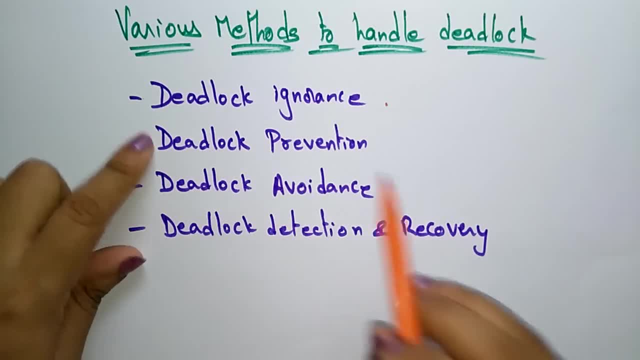 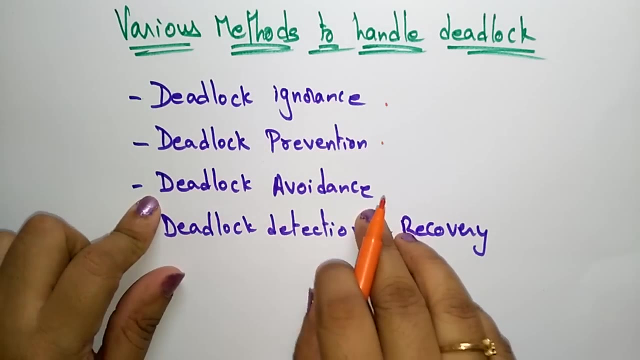 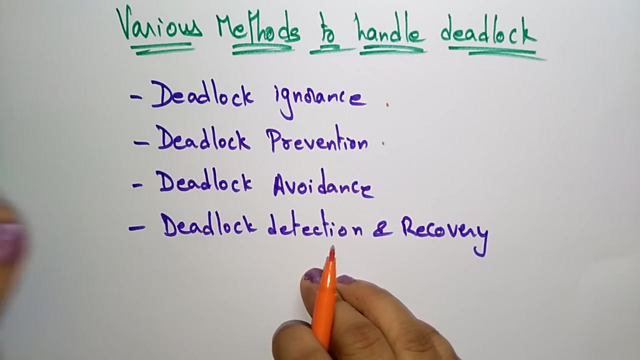 First thing is: try to ignore the deadlock if it is occurred. And the second thing is: it's okay if deadlock is occurred. According means: try to prevent the deadlock before it reached the complete deadlock state. Try to prevent the deadlock, or else better, to avoid the deadlock. And next is suppose: if deadlock is detected, even though you try to prevent, even though if you try to avoid again it comes, the deadlock is detected. So 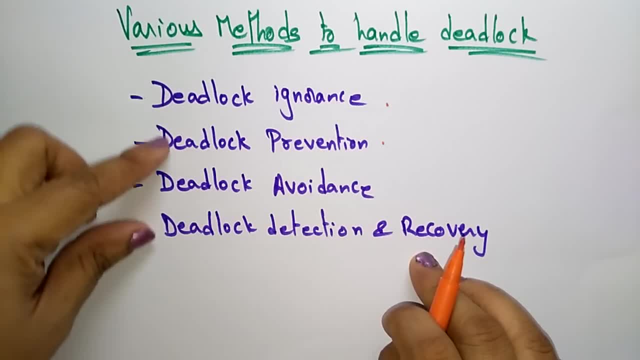 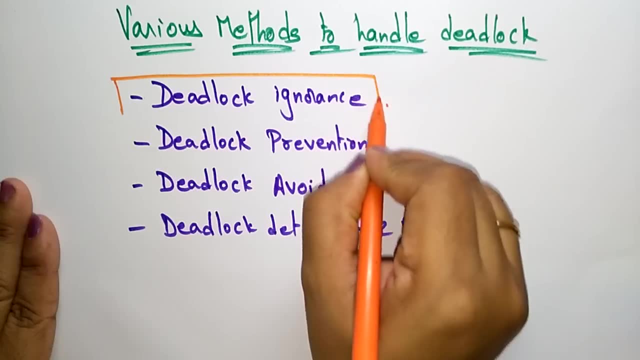 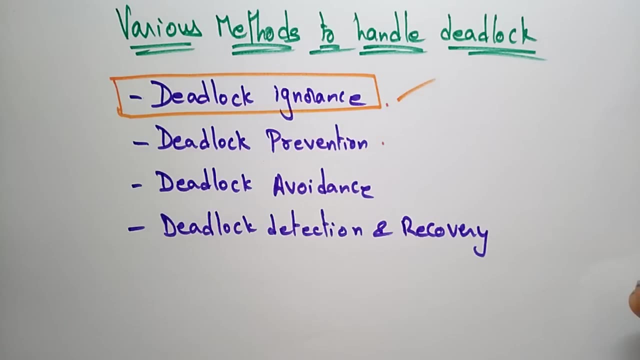 Most people try to recover the deadlock, So these are the different, various methods that are used to Whenever you try to recover it. first, let us discuss the first thing, that is, the deadlock ignorance, how we are ignored the deadlock, So actually. so again, Deadlock. I said It is a state when the two or more process or trying to access the same resources. 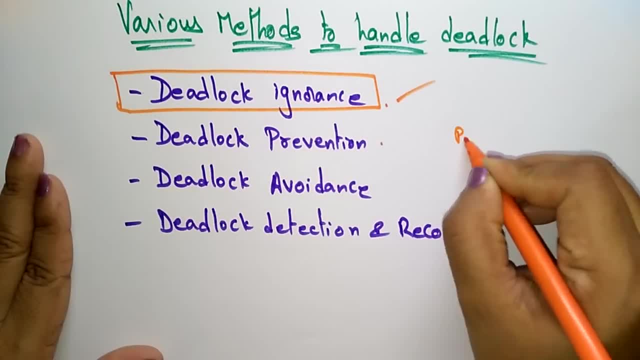 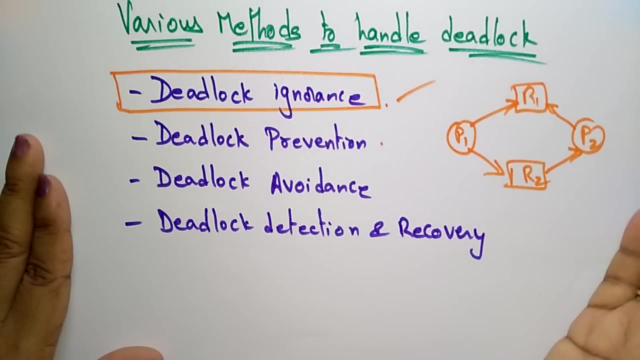 then a deadlock may occur When, When Process P1 is accessing the resource R1 and requesting the R2 resources and the process P2 is accessing R2 resources and requesting for the R1. Means, this is a deadlock state. a deadlock will occur. 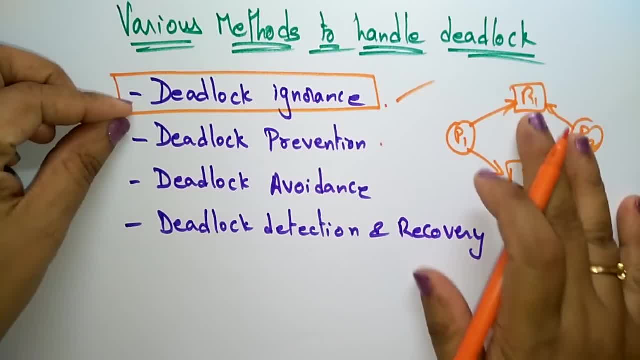 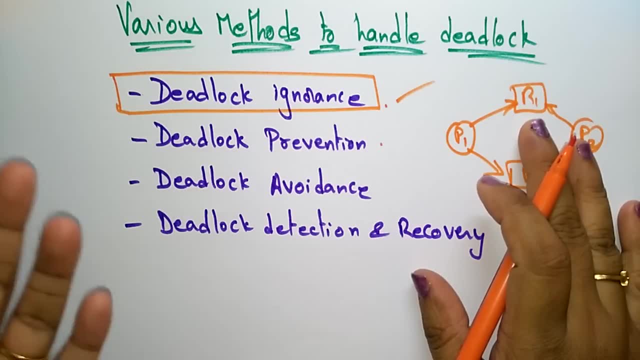 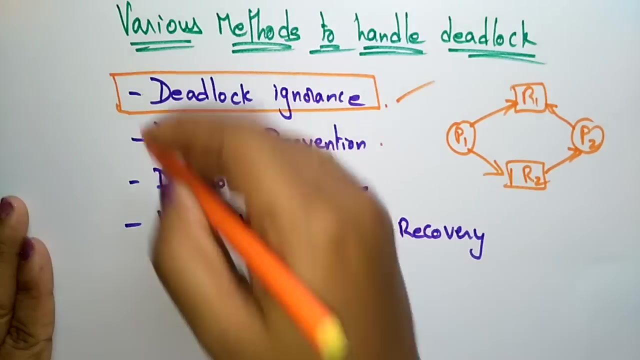 So better to ignore the deadlock. that is the first case. So you may get the doubt: if you ignore the deadlock, is there is any problem If you just avoid the deadlock? if there is any problem that exists, So just ignorance of deadlock, which will done by whatever the operating systems- mostly used operating systems like Windows, Linux and different mostly used operating systems- or try to avoid the deadlock. 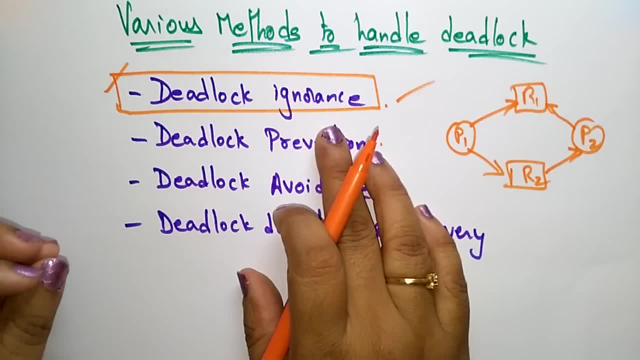 Means: try to ignore the deadlock, not avoid. try to ignore the deadlock. Okay, you may get the doubt. okay, the Windows operating system is ignoring the deadlock. Is there any problem if it ignores? Actually, the deadlock will occur rarely. 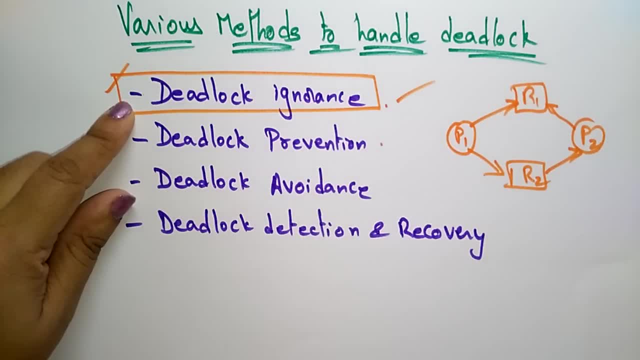 Only in the rare conditions it occur. So whenever it occurs the operating system will hang. So suppose if you are using the Windows operating system, whenever your Windows operating system are using, suddenly deadlock is occur. Means a same resources wants to access the multiple process. 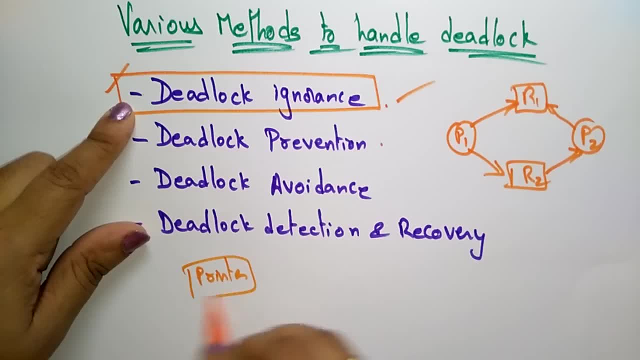 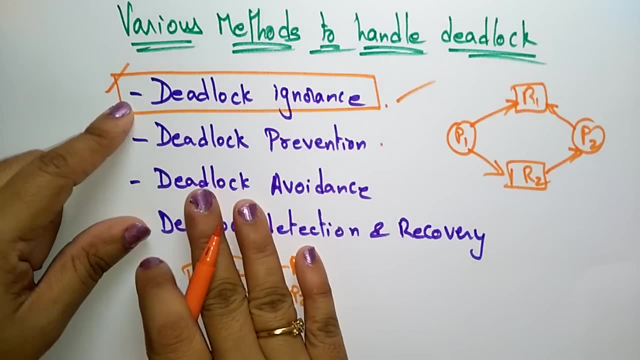 A printer is there. the printer wants to access the multiple resources process P1 and the P2.. Okay means multiple resources want to access The printer at the same time. Then a deadlock will occur. So whenever the deadlock will occur, your operating system will hang. 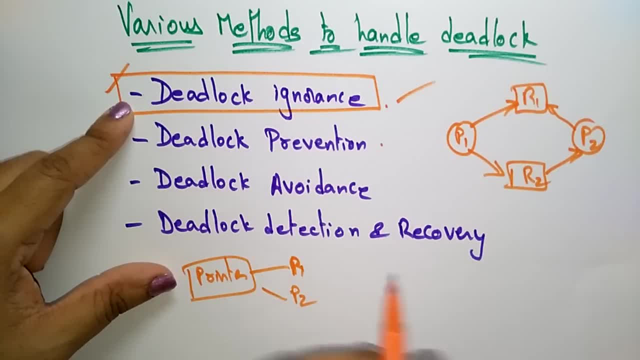 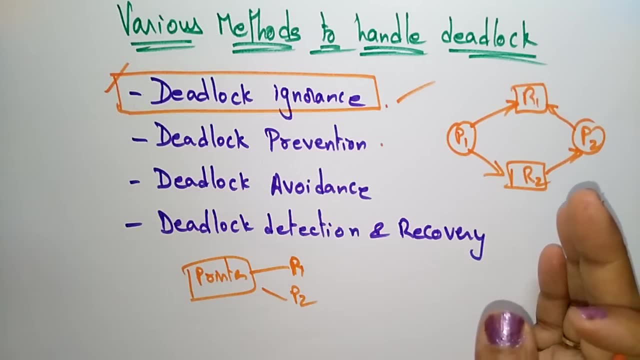 So what do you do if? if your operating system hang, what do you do? You just restart your system. So whenever you restart your system, that problem will be rectified. So writing that is that you call it as a deadlock- ignorance. 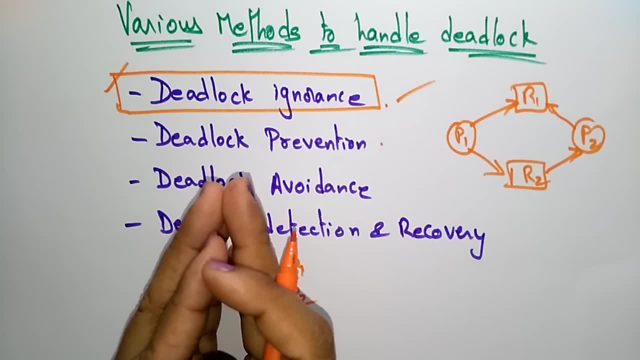 Try to ignore the deadlock If there, if you're dying deadly, deadlock is occur in your system. If there is a deadlock, a deadlock is occur in your system, system. try to ignore just by simply restarting your system. so that is the main. uh, it's a best. 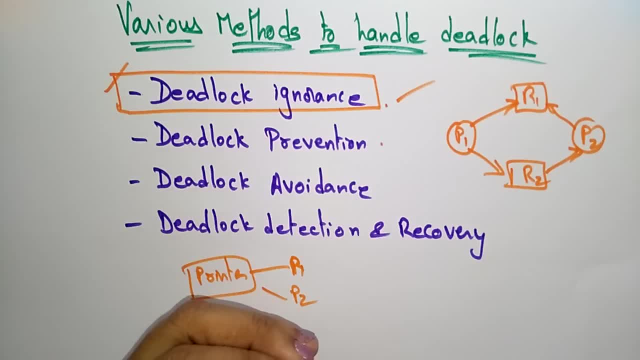 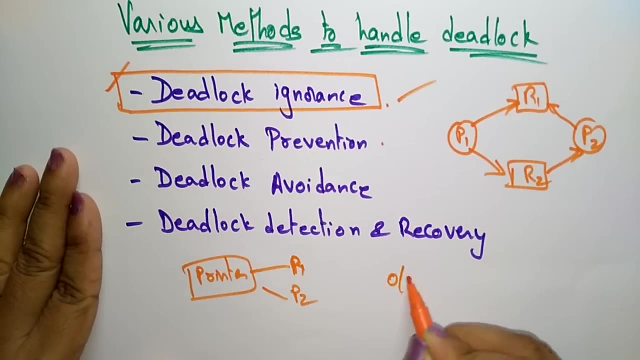 solution for operating systems. okay, you, you'll get a doubt that. okay, why we are ignoring the deadlock. it's better to write the code. if you write the code, your system will increase your system performance. you may get the doubt. so actually your operating system is having so. 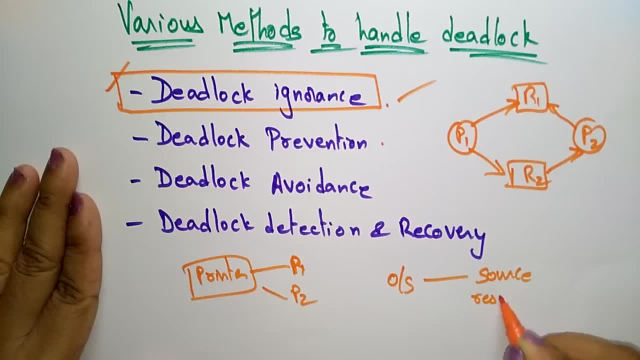 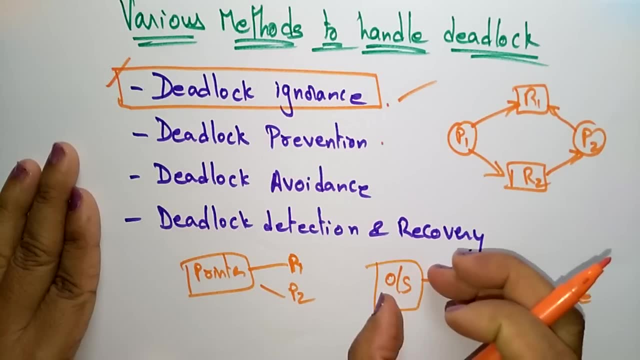 much of source code, source or resource code. so so much of resource code is already available in your operating system, a software code suppose. if you want to add, add deadlock code. if you want to add a deadlock code to this resource code somewhat, a burden will be increased. 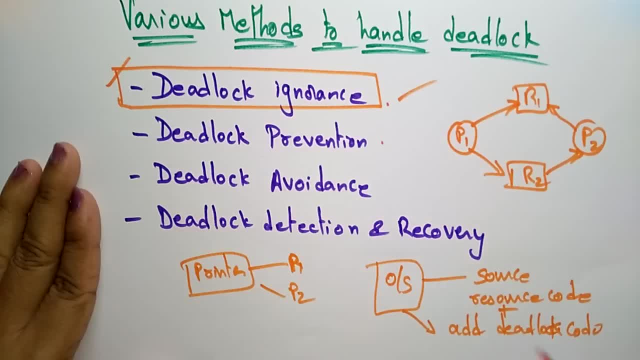 means every time the system, whenever you start the system, this deadlock code operates so much of source code, so much of resource code is already available in your operation is also monitoring means it is also performing the operations. it also uh restart every time it is uh completely reading the. the operating system is reading complete code of the. 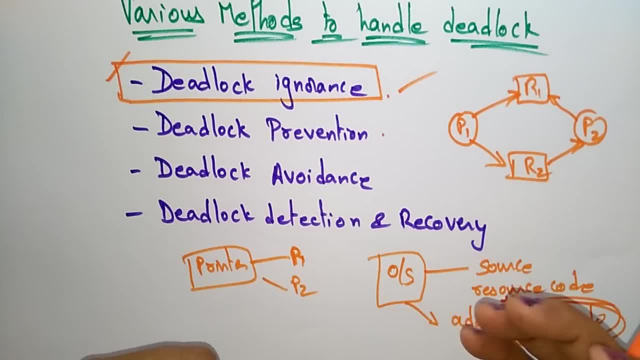 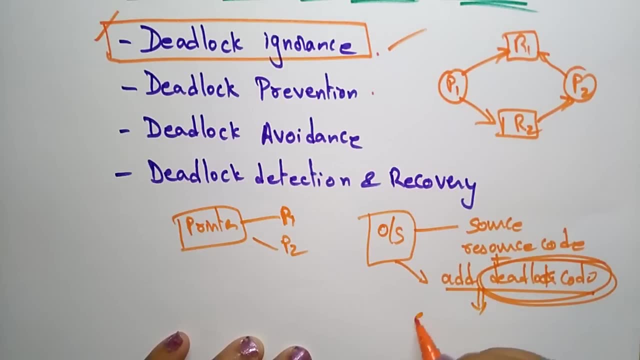 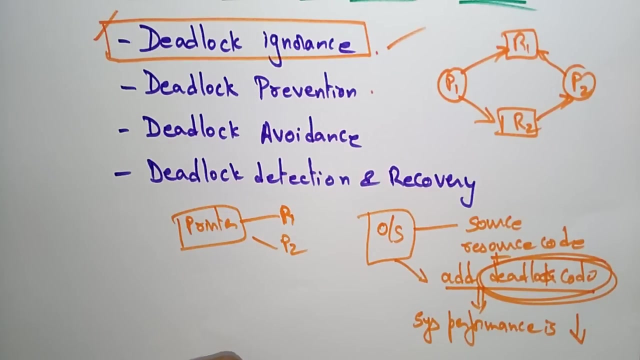 deadlock also, even though it is not required. so obviously your system performance is decreasing whenever you add the deadlock code to your operating system. system performance. performance is decreasing means the speed is decreasing and the capability of your system is decreasing whenever you add this code to your resource code. okay, so it's better to. avoid. it's better to ignore that code, suppose. if you just ignore this deadlock code, okay, so then your system and then your system capability will be increased, capability will increase, okay, and the system speed will be increased and system performance will be increased. so rather, it's a many advantages if you didn't add the deadlock code to your operating system. 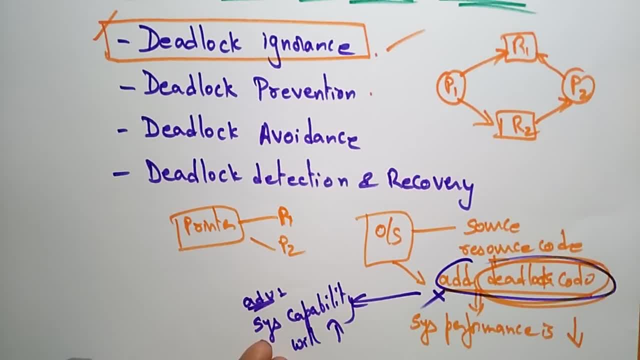 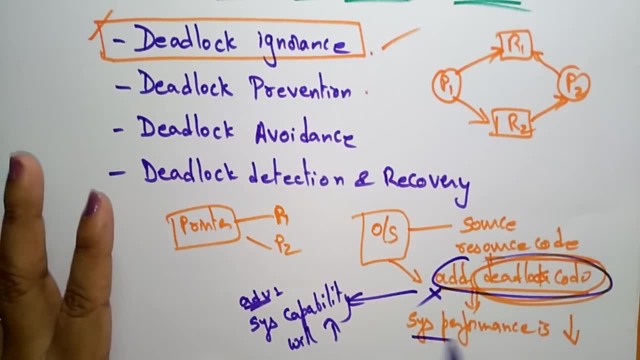 you have so many advantages, your system performance will be increased. suppose if you add a code to your deadlock. deadlock may not occur to your system, but your system performance will be decreasing. so the main aim of your our thing is that we want to use the operating system which is so efficient. 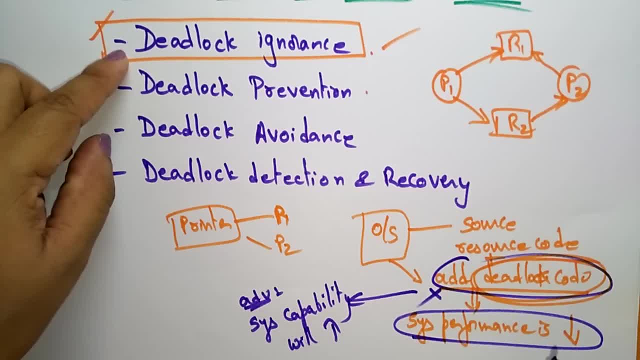 okay. so a deadlock may occurs rarely. so for occurring the deadlock code you have to use a deadlock rarely. if you add the code to your operating system, your system performance is decreasing. so to avoid that decreasing the system performance, we are not adding the deadlock code in in our operating system resource code, operating system software so that the system capability and the performance will be increased. okay, so whenever you occur the deadlock, just try to restart your computer. that is a main solution and the only solution for your windows or linux operating systems to avoid this, to ignore the deadlock. so if you want to ignore the deadlock, just restart your. 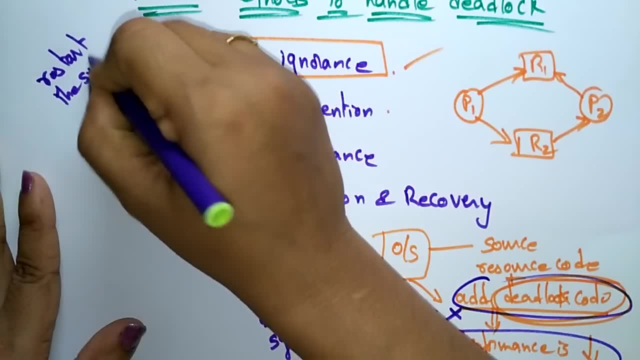 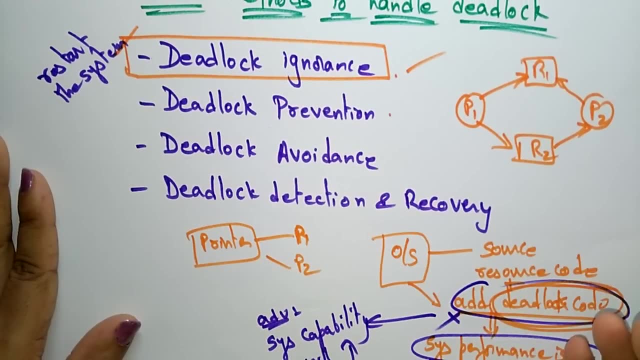 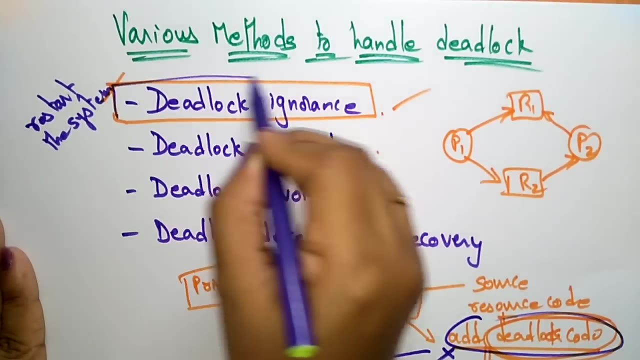 system, restart the system. so this is the better solution to make that so, rather than adding the code, your operating system and making your operating system performance decreasing, your system performance is decreasing better to restart the system. so this you call it as a deadlock ignorance. so nowadays, every system, whatever the system you are, you're taking the operating system.